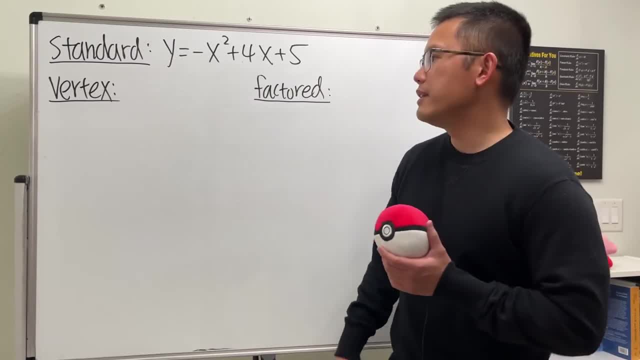 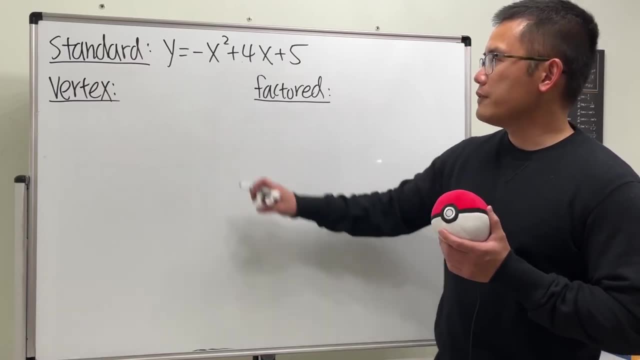 When we are given the parabola in the standard form, how can we write it in its vertex form and also in its factorial form? Well, this is our example, and let's see what we can do. First off, the standard form says the coefficient of x squared is going to be the a value. so that means: 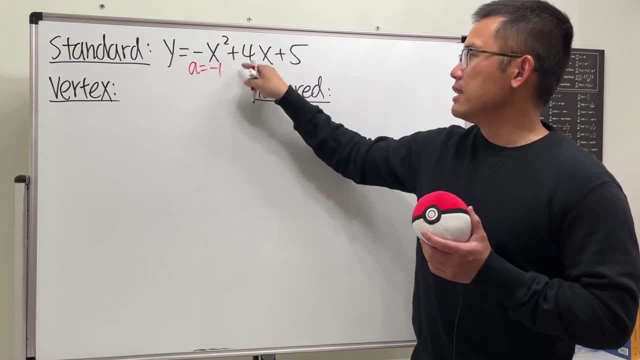 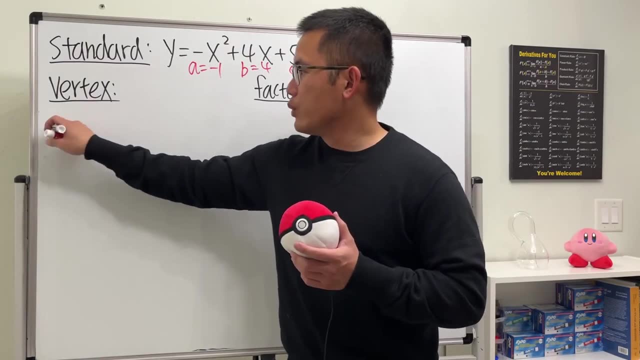 we have negative 1.. So let me indicate that for you guys. And then this is the b value, which is 4, and c is equal to 5.. Let's get the vertex first. This right: here we will use the vertex formula. 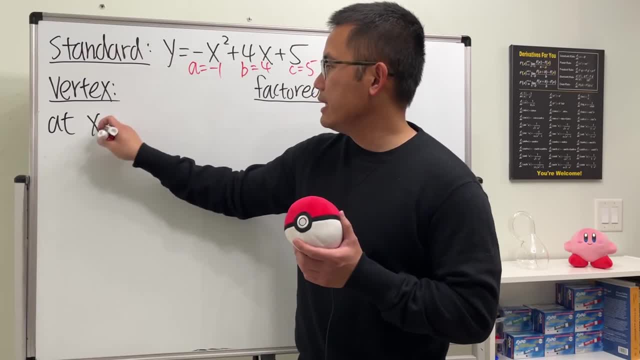 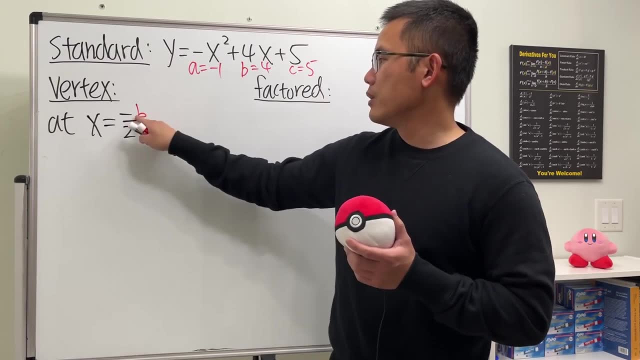 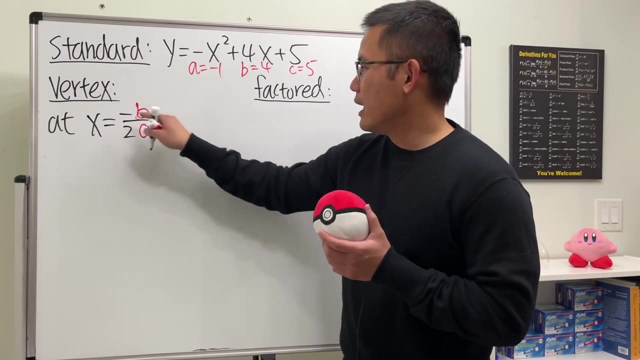 and it says the vertex will be at: x equals negative b over 2a. So this is just a little formula that we can utilize, because we're given the equation in the standard form And then let's just work that out Here. we have negative and then the b is 4, and then we have 2 times a. 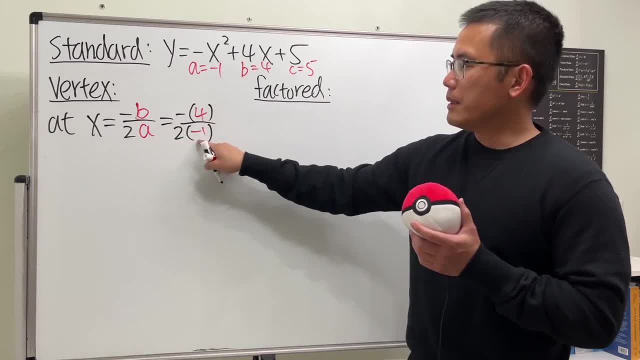 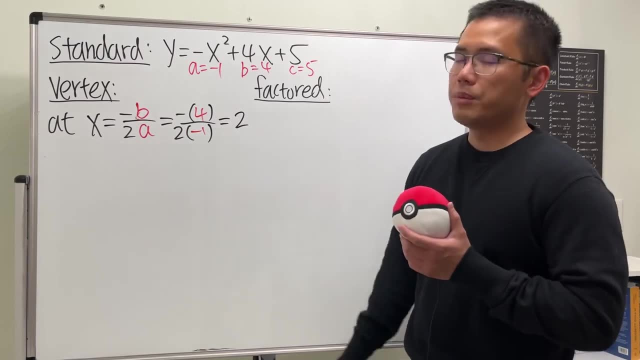 a is negative 1.. So 2 times negative: 1 on the bottom is just negative. 2. Negative 4 is negative 1 on the bottom. So 2 times negative 1 on the bottom is just negative. 2. Negative 4 over negative 2, we will get positive 2.. So that will be the x value. 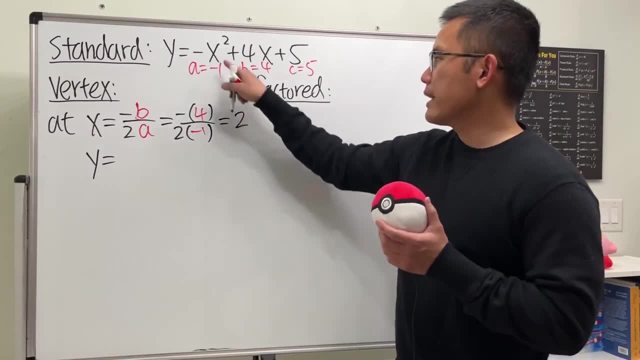 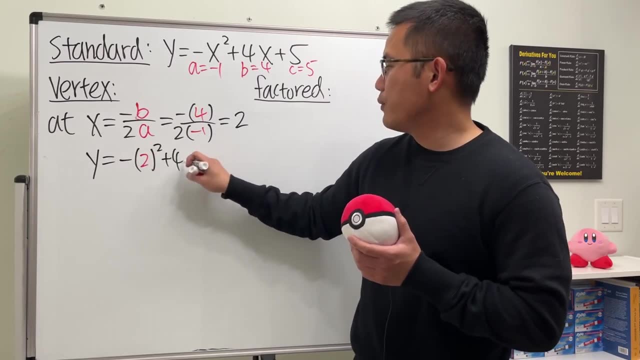 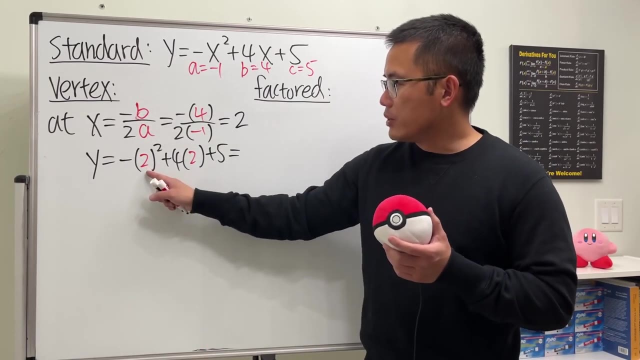 Then we are going to compute the y value by plugging this back to this x and also the x. So we will have negative parentheses, 2 squared, and then plus 4 times 2, and then plus 5.. So let's work this out real quick. This is 2 squared, You do that first, which is 4,. 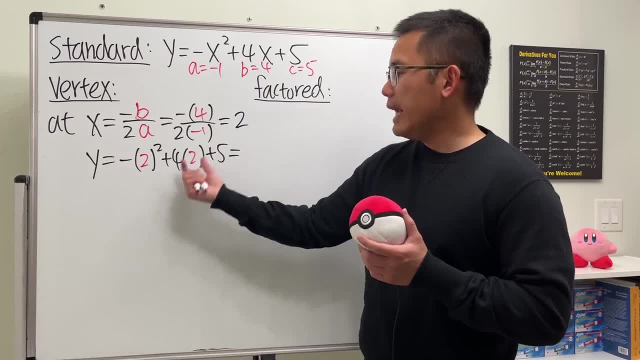 and then you have negative 4 here, right, Negative 4 plus 8,, which is positive 4, and then we add a 5 to it, which is going to be 9.. So this is 9,, all right. 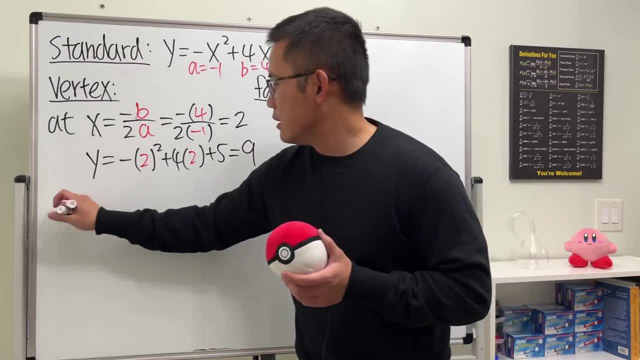 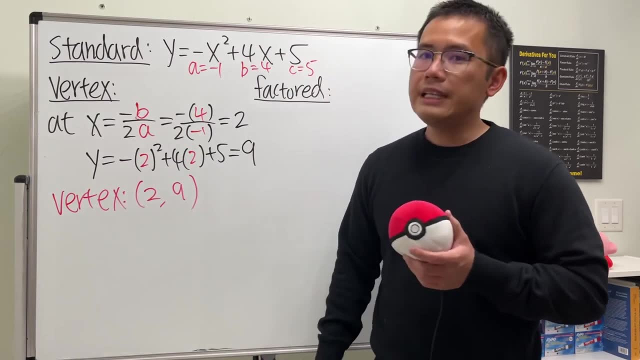 So we know the vertex is 2, 9.. So let me just write this down here for you guys: Vertex is 2, 9.. And in fact, once we know this, we know this is the h value and also the k value here. 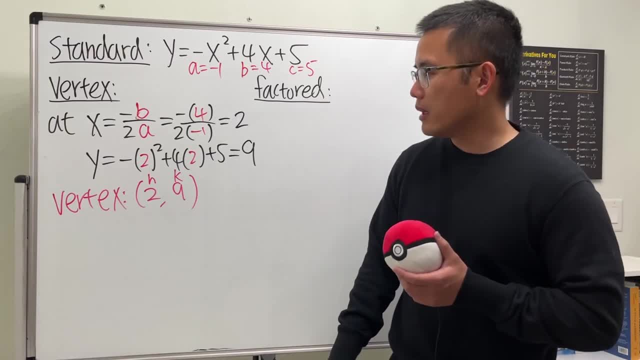 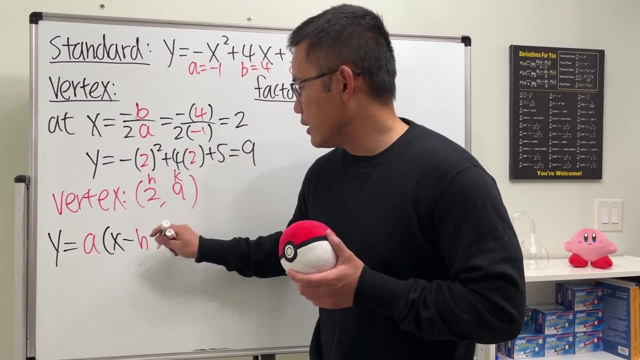 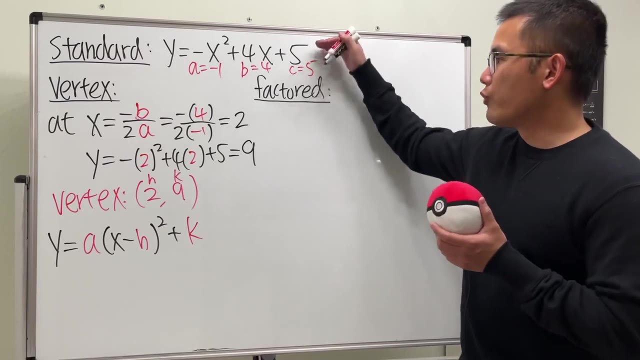 in the vertex form of the parabola. So the vertex form is this: y equals a times x minus h and you square that and then you add k to it. You can also do the completeness square technique to go from here to here. 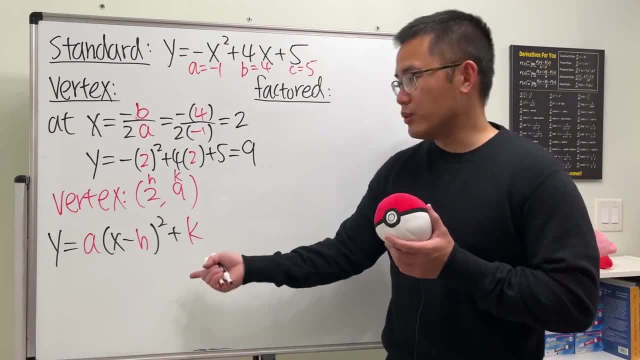 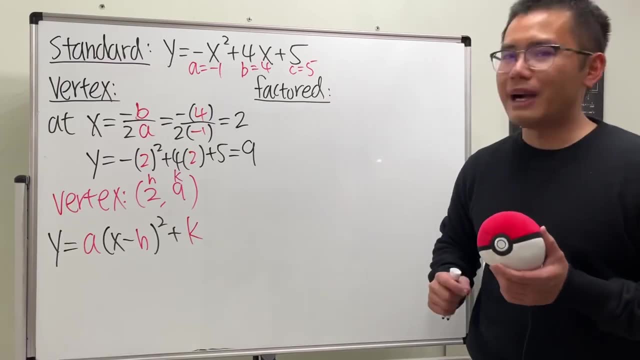 but seriously, if you really just want to get into the vertex form, compute the vertex like this and then plugging. I think it's much easier, And that's what the teacher says. You have to do it by completing the square. 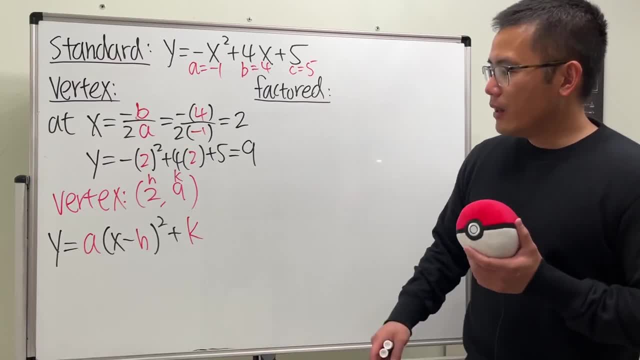 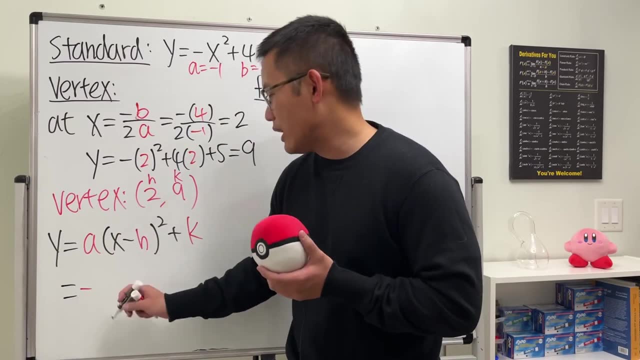 then you follow the direction, But this is totally okay, All right. where's a? Well, it's the same a right here. So in fact we will have just negative 1, and it's just negative, You don't have to put on the 1.. And then we have x minus h, which is 2,. 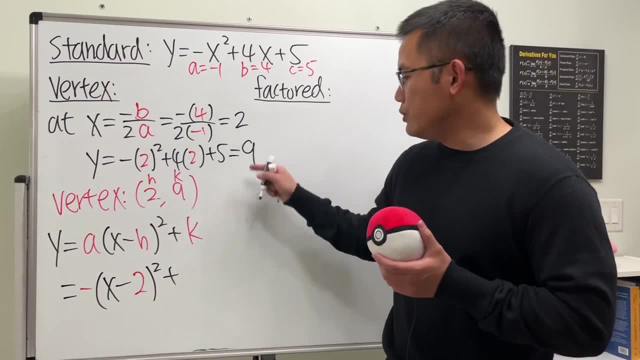 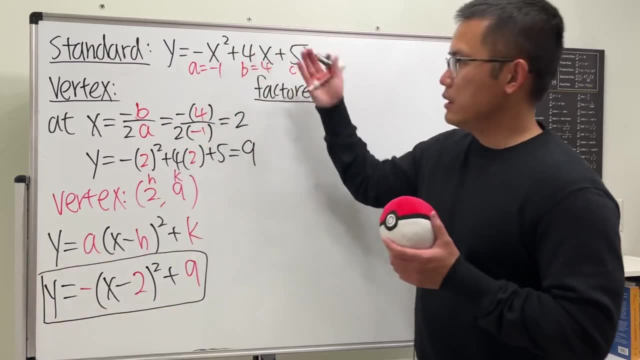 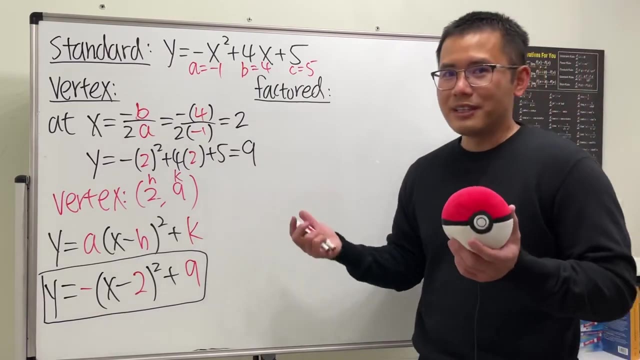 and then we square that, and then we add a k, which is 9.. So, ladies and gentlemen, this, right here, is the equation in the vertex form. all right, Cool, Now let's look at the factored form. So, by the name, he suggests that we just have to factor it. And for the factored form, 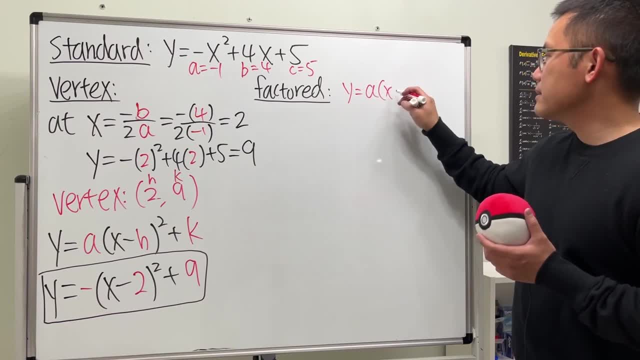 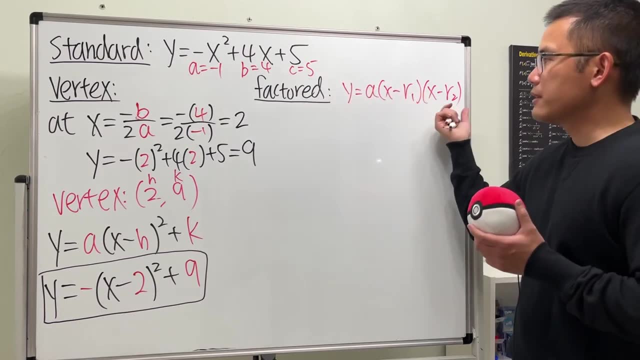 it's going to look like this: y equals a times a x minus r1, times x minus r2.. You see we have the expression being factored in and then we actually have the same a. all right, And I should have put down the vertex form, right. 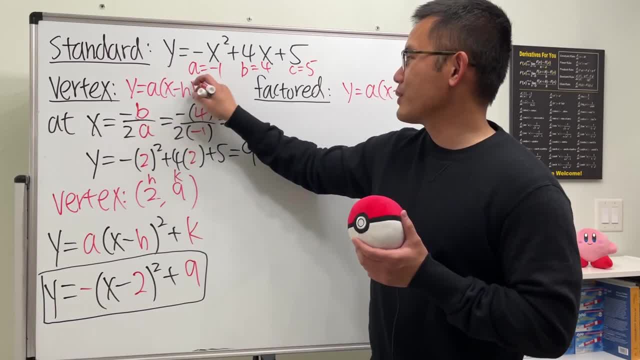 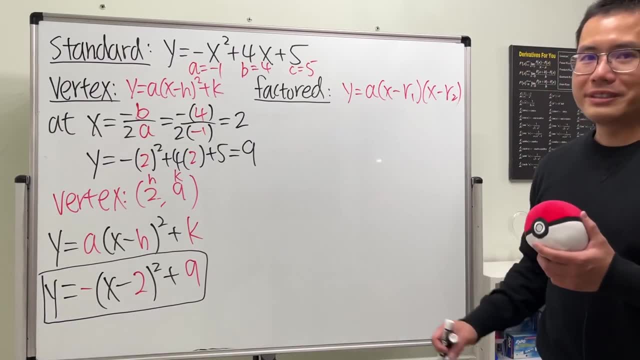 here for you guys. first. So y is equal to x minus h, squared plus k. Let's just keep it like that. I've already done over there, though, Anyway. so how can we do this? Well, just go ahead and factor it, and then you preset it in the factored form. Here is our original. 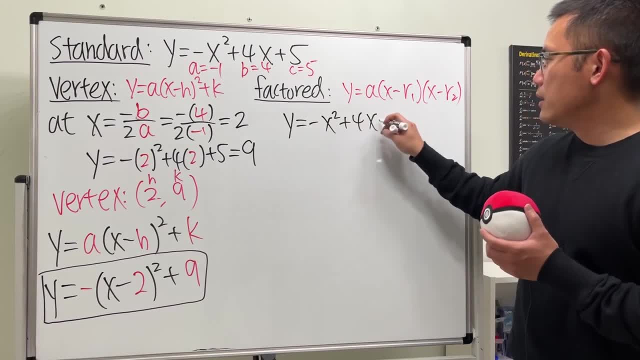 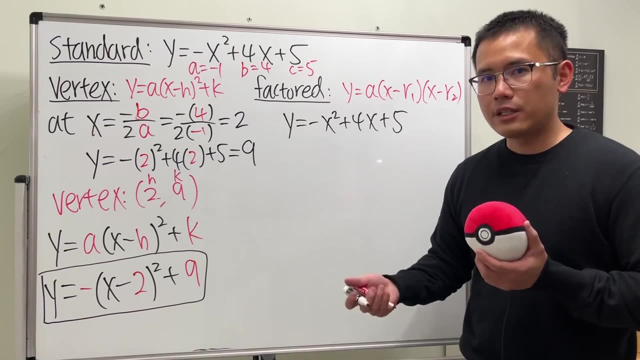 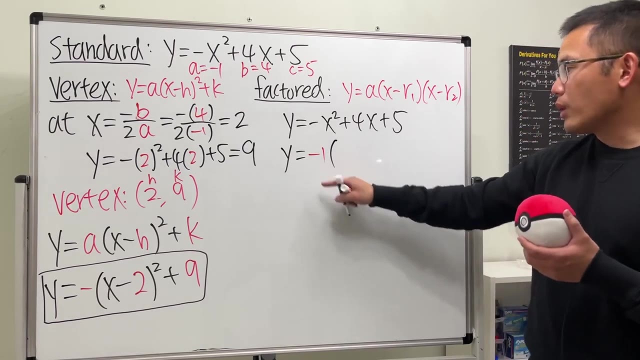 in the standard form. Well, we have a negative in front of the x squared. So the first step is technically to factor out negative 1. So y will be equal to. let me factor out negative 1.. Put this down on purpose: negative 1.. Originally this is negative x squared. 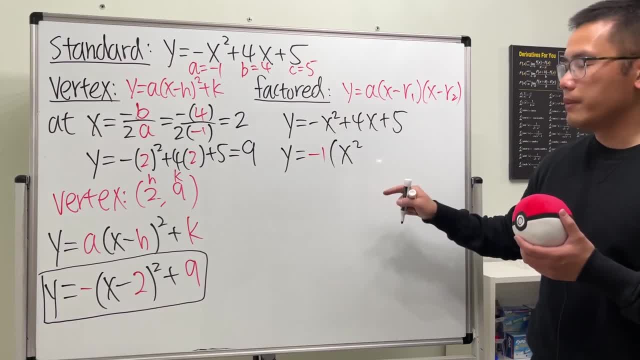 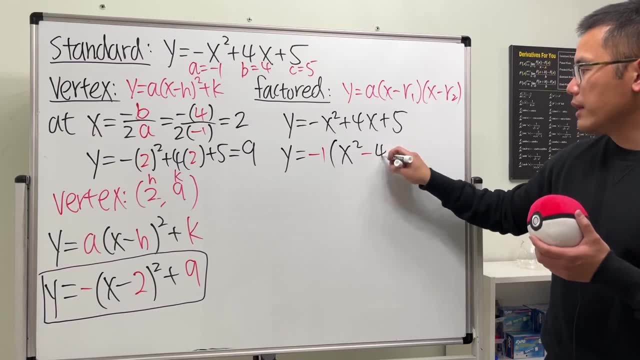 but we factored out negative, so this will be just positive x squared. Originally this is positive 4x, but we factored out the negative, so this will be negative 4x. Similarly, 5 was positive, but we factored out negative, so this will be negative. 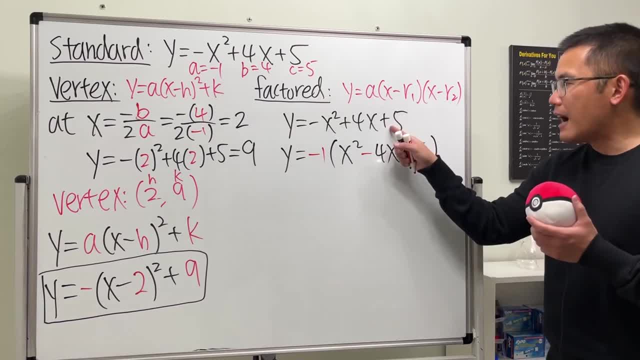 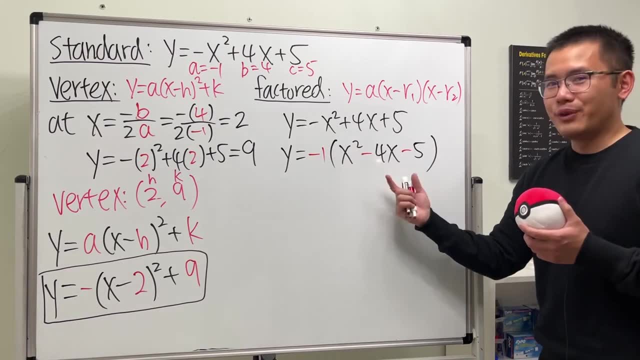 Or, if you would like, you can also think about this as division: 5 divided by negative 1 is negative 5.. Negative- sorry- 4x divided by negative 1 is negative 4x, et cetera, et cetera. 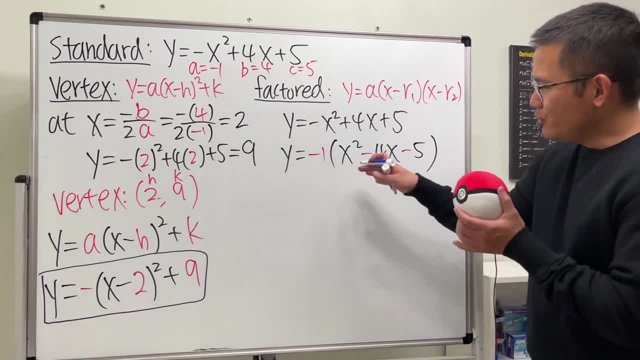 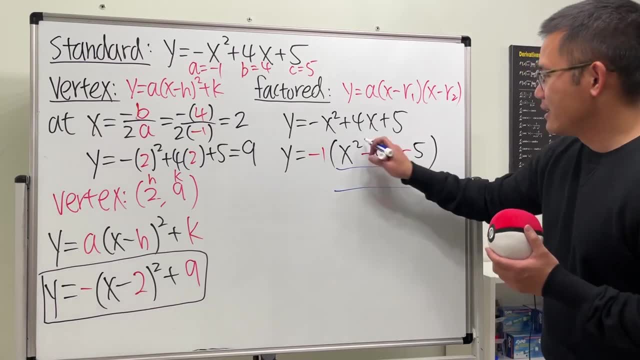 Now, how do we do this? You might be able to just eyeball it, just look at it and write down the answer. That's totally okay. but I'll show you guys the tic-tac-toe method. Because why not? x times x gives us x, squared Perfect. What times 4 gives us negative 5?? 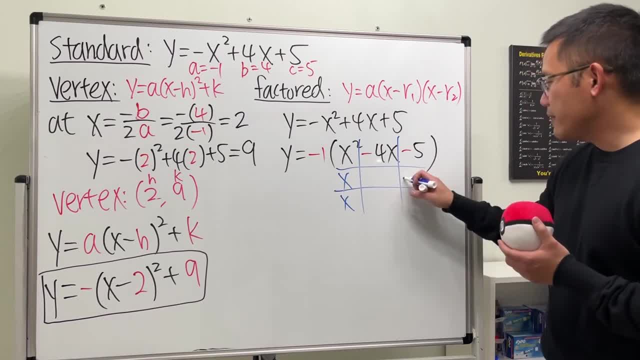 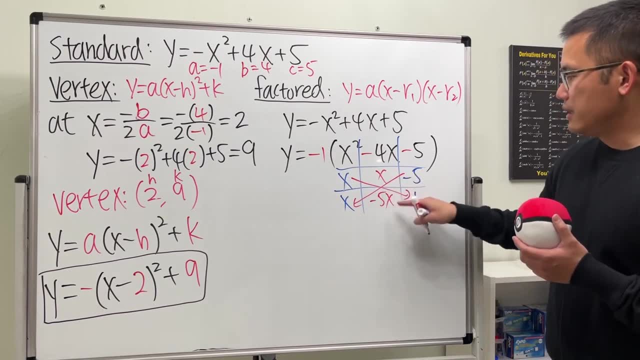 Together they have to add up to negative 4.. Just negative 5 and 1.. How's that? You see, this times this is x, This times that is negative 5x Together. we do end up with that. 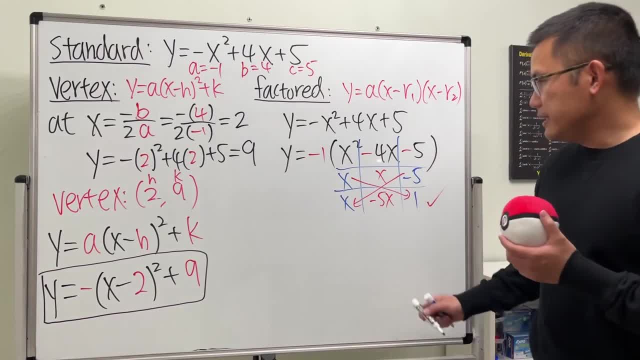 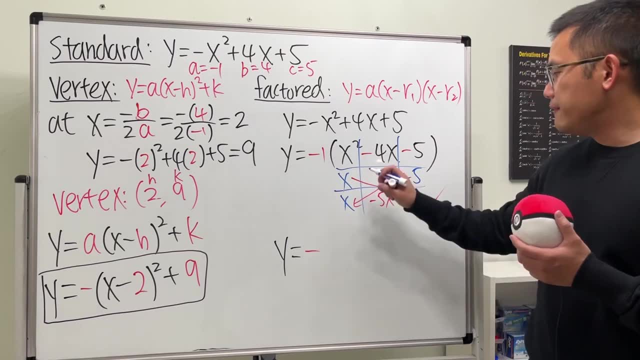 so we know this right here is correct. So, ladies and gentlemen, y equals. here we have the negative 1, but we can just write down negative like this, And then the factor for this is: remember to read it across. So we have x minus 5. 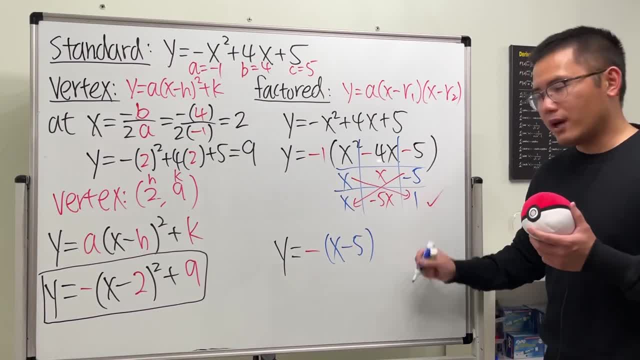 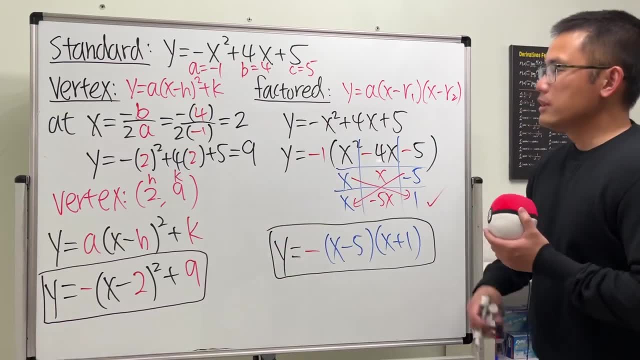 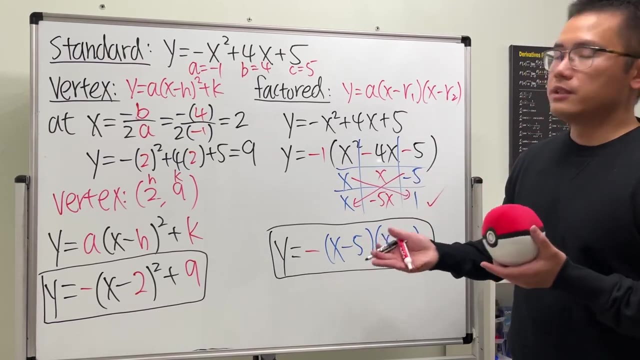 times x plus 1.. So let me just write that down here, Cool, And then we are done, right. So that's the question. But you know, once we have this and that, in fact, we will be able to make a graph of this real quick. So let me just talk about it right here. 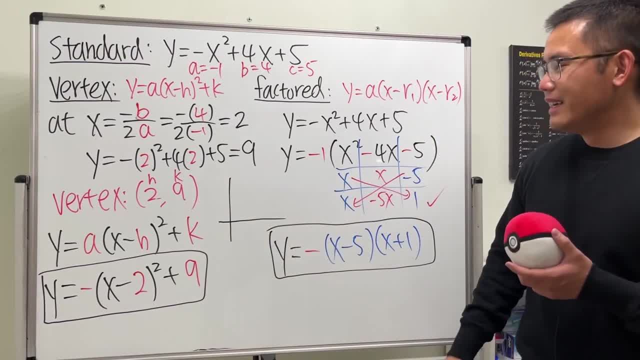 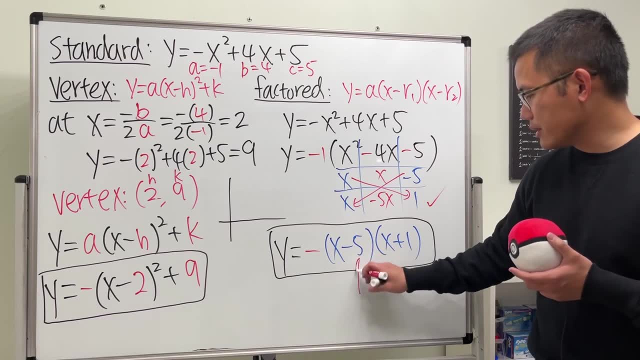 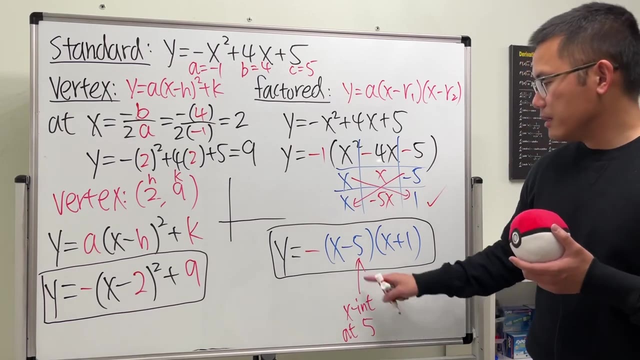 This is like a little bonus part. Okay, When we have this x is well, this right here tells us: you know, like this right here tells us the x-intercept is at positive 5.. Because, you see, this is x minus r1.. r1 is 5,. 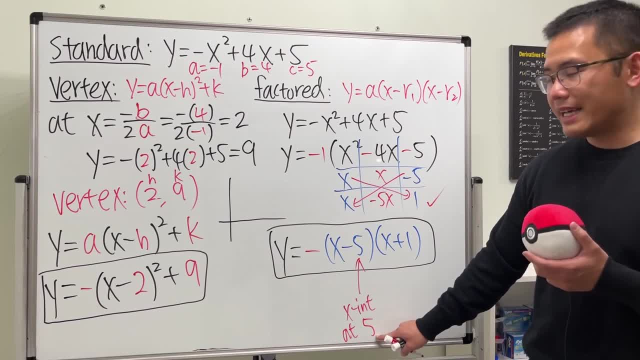 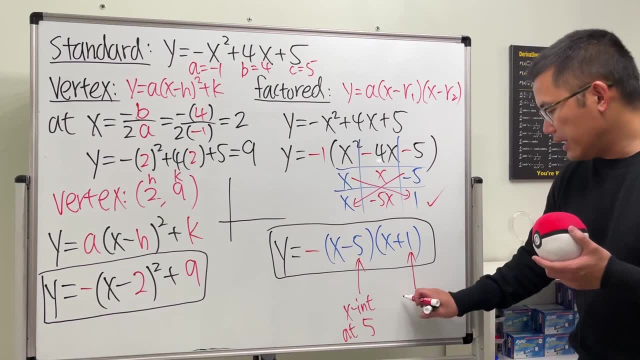 so it's just 5.. Or, if you would like, you can make this equal to 0, and you add a 5 on both sides, So that's why it's 5.. And then you also have x-intercept. it looks like it's positive 1, but no, You remember, you make x plus 1 equal to 0,. 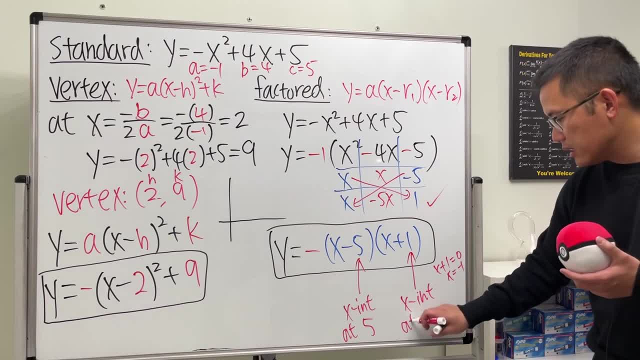 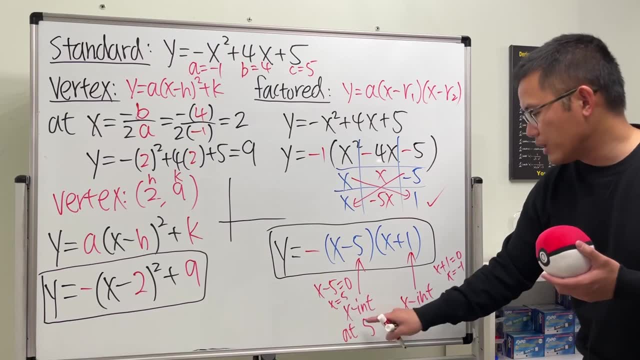 so x is actually equal to negative 1.. So it's at negative 1.. And again this right here: x minus 5 equals 0, x is equal to 5.. So we have this and that. So right here, I will just say this: 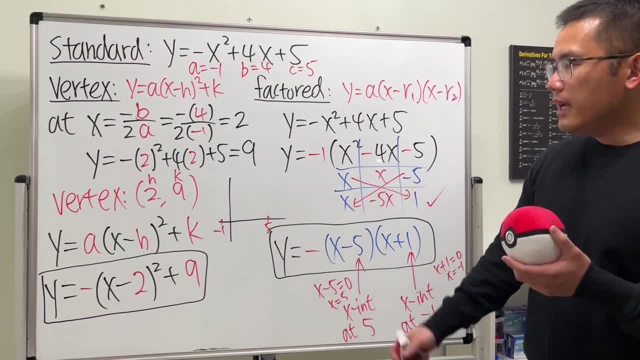 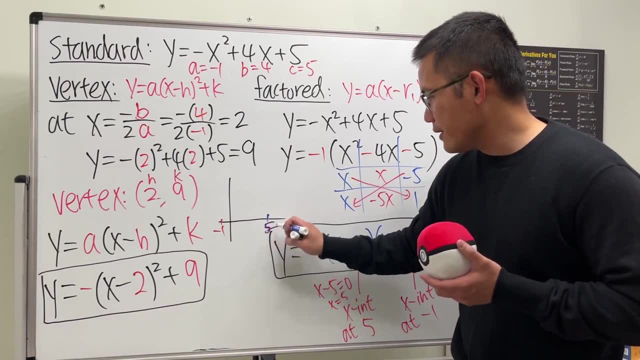 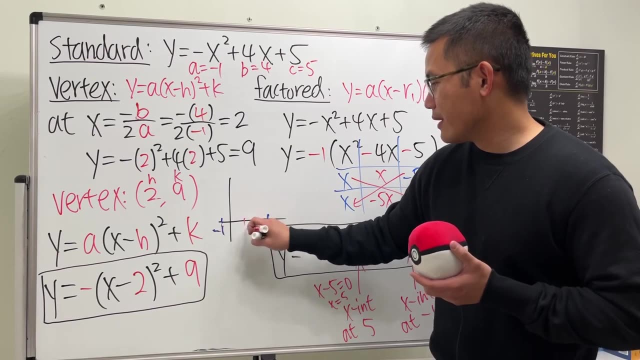 is 5, and this is negative 1.. Okay, And then we also know the vertex, which is 2,9.. So perhaps I'll put this down. Well, actually I'll put this down in blue. This is the 5,, and now that's purple, The vertex is 2,9,. so let's say here: Check this out. 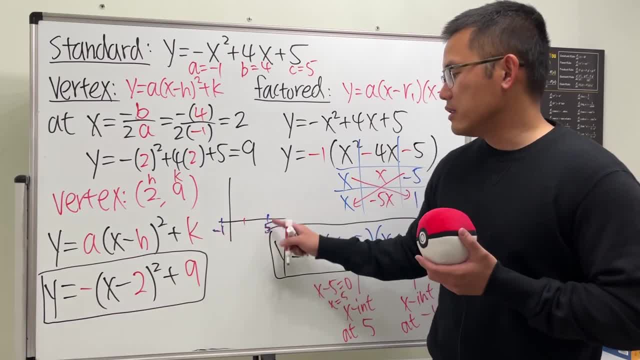 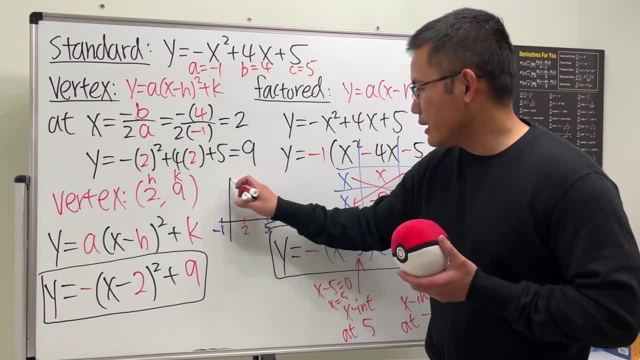 The vertex is always going to be in the middle of the x-intercepts. Yeah, that's a beauty, Because it's always symmetrical when you have a parabola. But anyway, here's 2, and then let's say: here is: 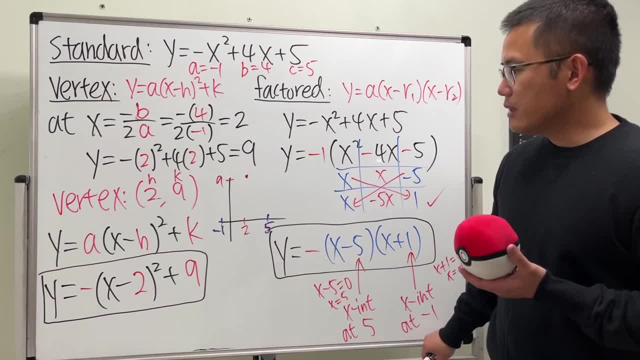 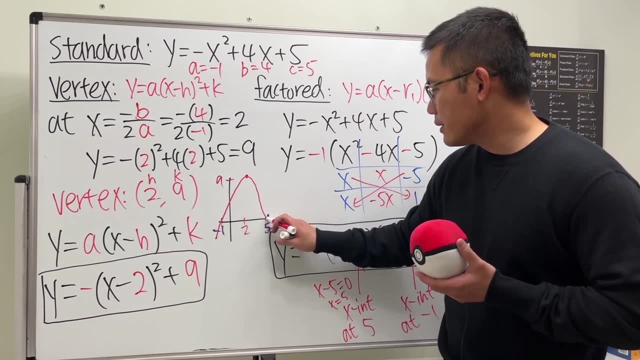 the 9,. so you have the point here And, as you can see, we can just go ahead and connect the x-intercept, the vertex, and then another one somewhat like this. Let me just make it better for you guys. 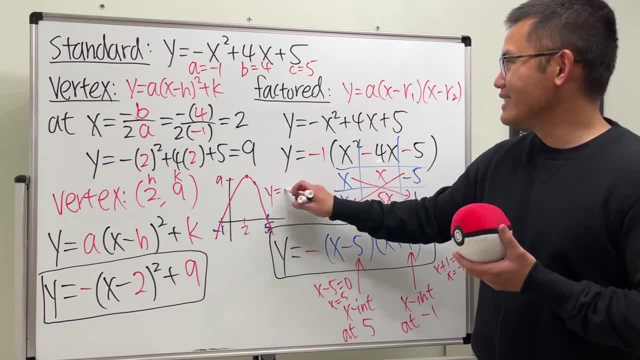 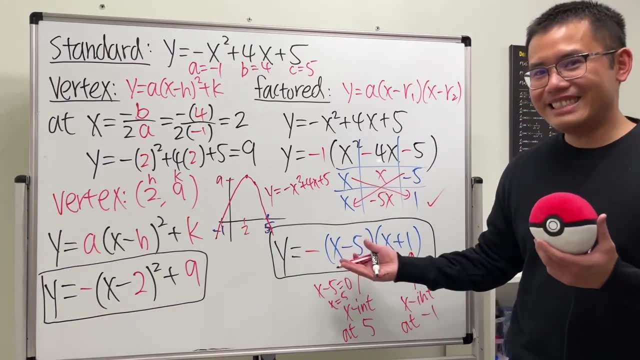 Yeah, So this is the graph for that. y equals negative x squared plus 4x plus 5.. All right, So that's a little bonus part And that's it. You want a five inch thick layer of topsoil for a new 35 foot by 24 foot garden. The dirt store sells by cubic yard. How many cubic yards of topsoil will you need to order? You can only order a whole number of cubic yards. 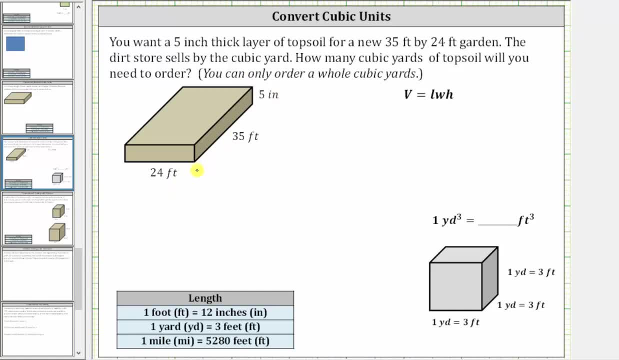 To begin, we'll find the volume in cubic feet and then convert the cubic feet to cubic yards. Before we find the volume in cubic feet, though, we have to have the dimensions in feet. Notice how here the height or the thickness of the topsoil is in inches. 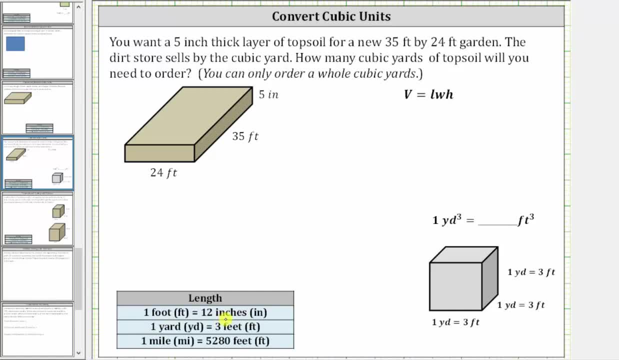 And since one foot is equal to 12 inches, one inch is equal to 1 12th of a foot, which means five inches is equal to 5 12ths of a foot. And now let's determine the volume in cubic feet.